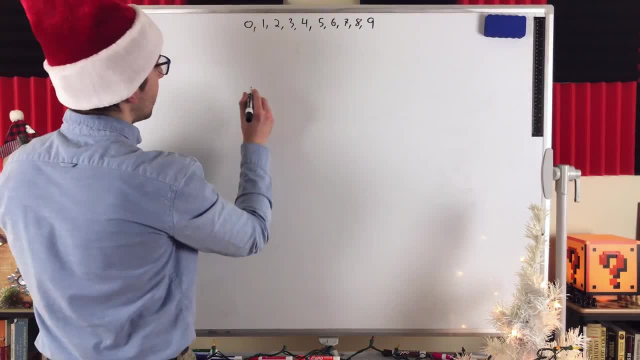 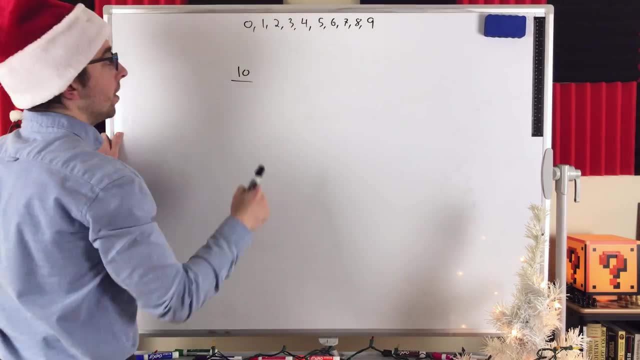 if we're allowed to use the same digit multiple times, Well, some number of our code has to be. first, Some digits got to go there. There's 10 total possibilities. any of these 10 digits? Then what about for the second number in our code? 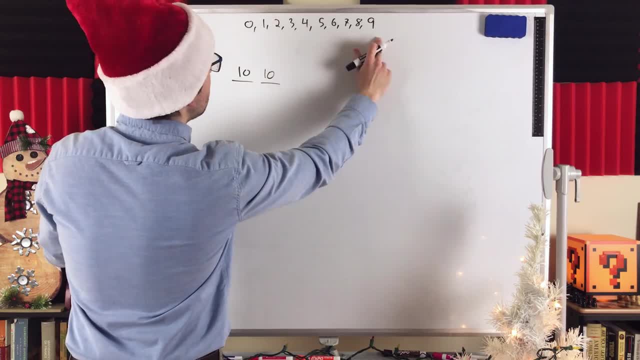 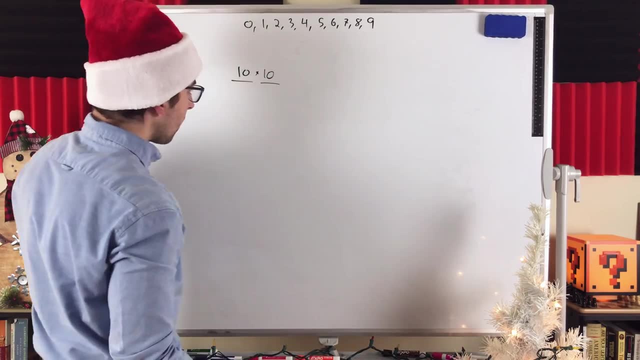 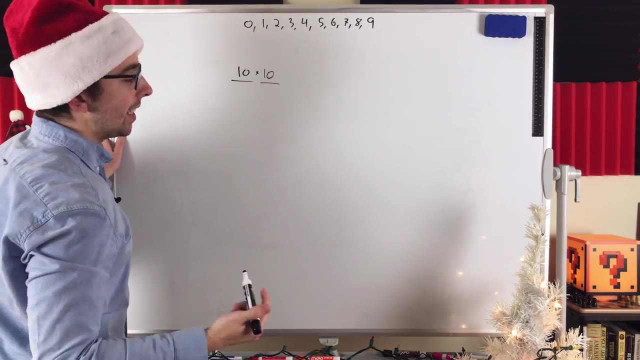 Well, there's still 10 possibilities, because we're still allowed to use any of those 10 digits. Now, to count up all of these possibilities, we need to multiply, Because for every one of the 10 digits that could go first, there are 10 digits that could go second. So we're going to need to. 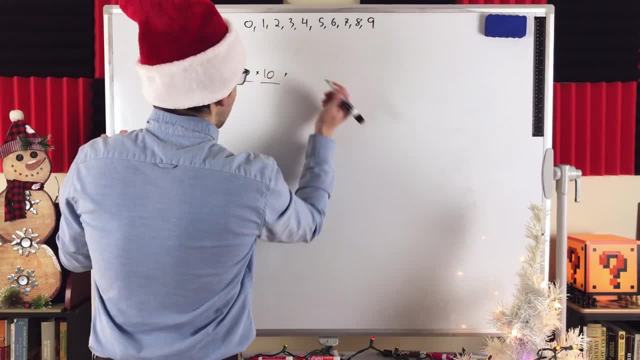 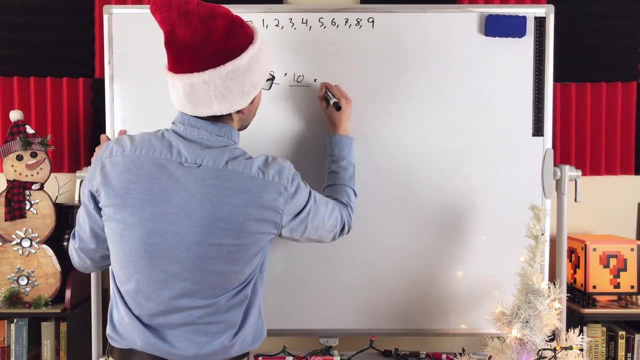 multiply to total up all those possibilities. Then same thing, It's pretty simple, for the third number. in the code There's 10 possibilities, any one of these 10 digits. Same thing for the fourth number, And so that's it. 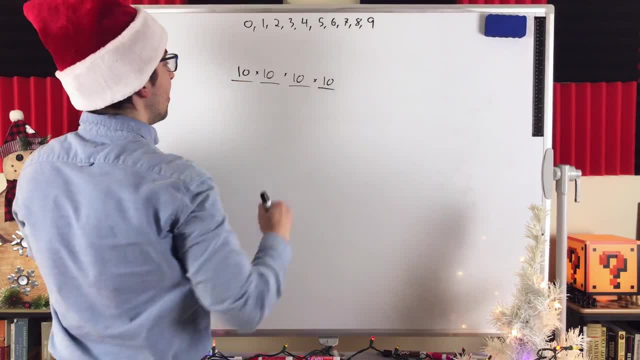 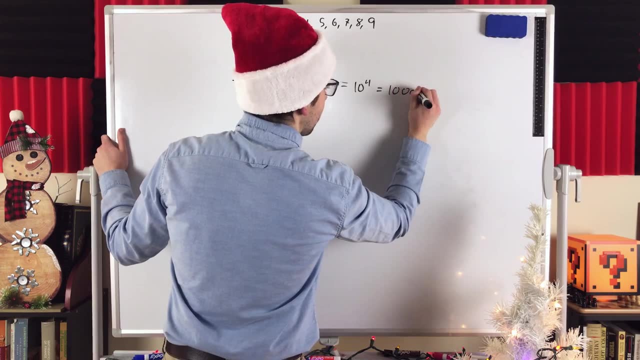 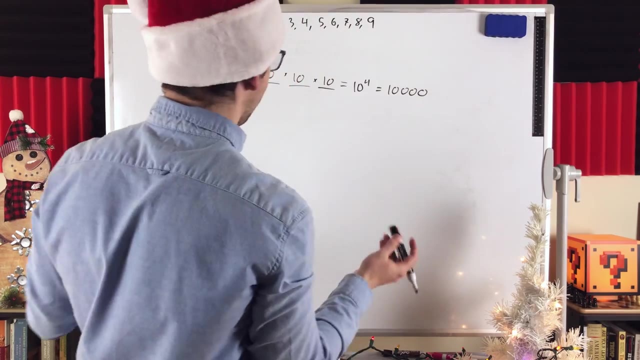 So the total number of four digit codes using the digits zero through nine and allowing repetition is 10 to the power of four or, if you prefer, 10,000.. You can use very similar reasoning to solve very similar problems. For example, what's the number of, say, seven digit codes using the 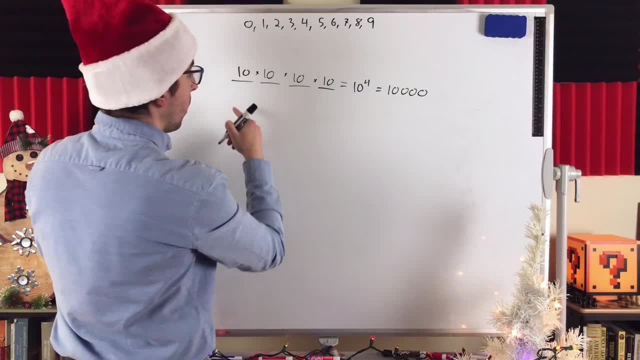 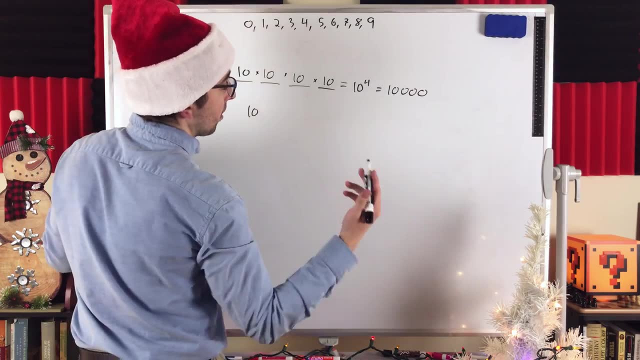 digits zero through nine and allowing repetition. Well, it's going to be the same thing 10 times 10 times, 10 times 10, but seven times because there's one, two, three, four. there's going to be seven total numbers in our code, because we're talking about a seven number code right now. 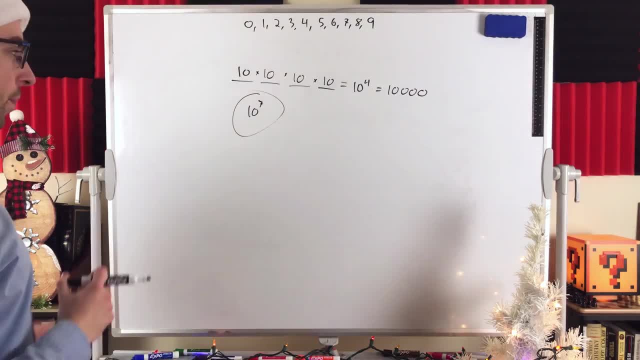 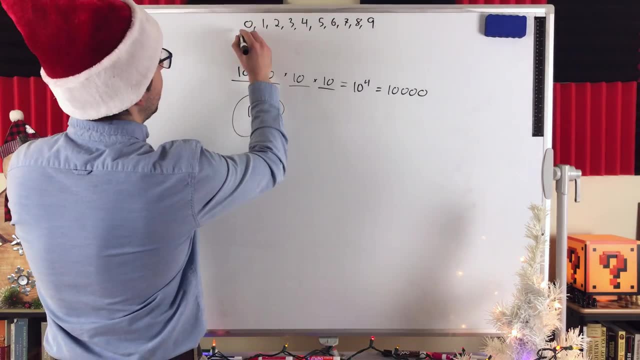 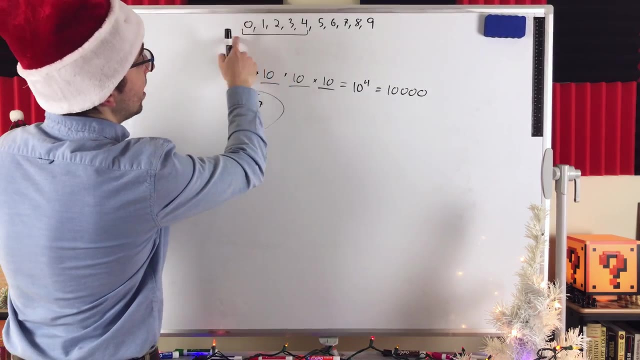 So the total number of possibilities would be 10 to the power of seven. Another similar problem would be: how many five digit codes are there, using the digits zero through four and allowing repetition. Well, how many digits are here? How many digits can we? choose from Zero, one, two, three, four, that's five digits. So how many five number codes can be created from those five digits? Well, that would be five to the power of five, because five digits can be in the first spot. 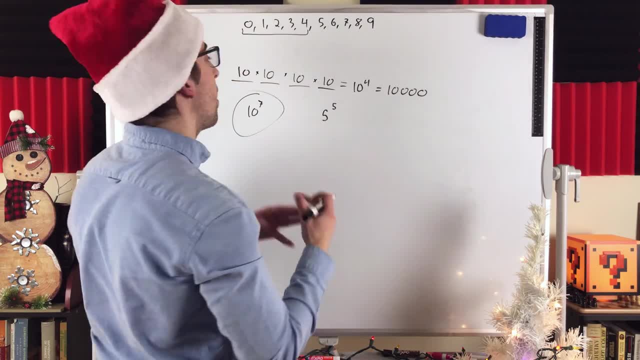 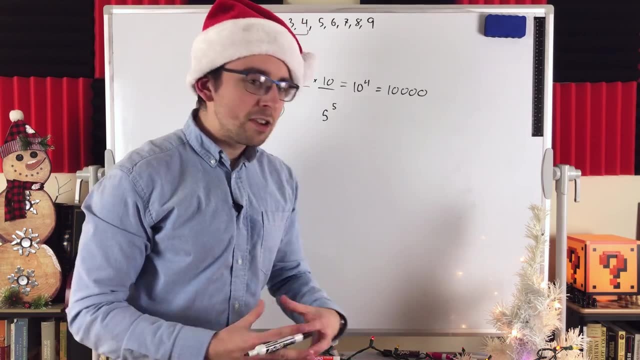 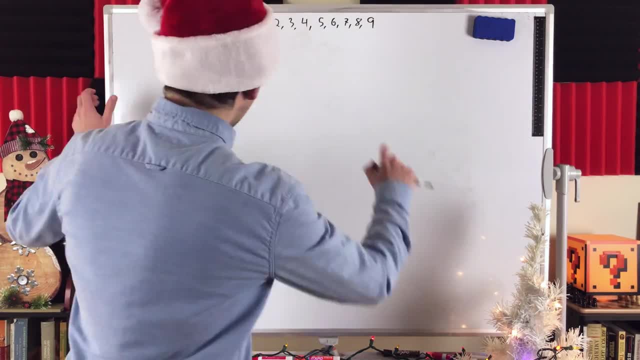 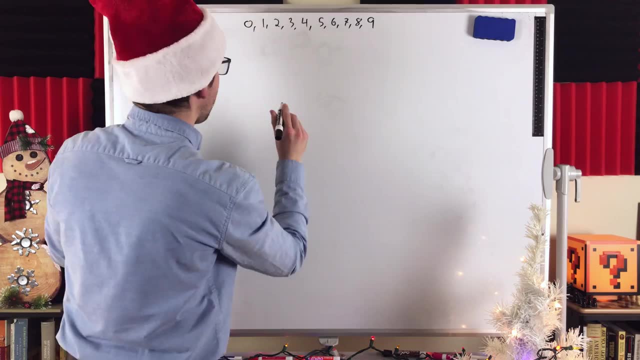 the problem to non-reasoning. So let's go ahead and switch the problem to non-reasoning, So let's go ahead. four number codes can be created using the digits zero through nine, not allowing repetition. It's a pretty similar problem, but it's got a bit of a different solution. Some digit has to go first. 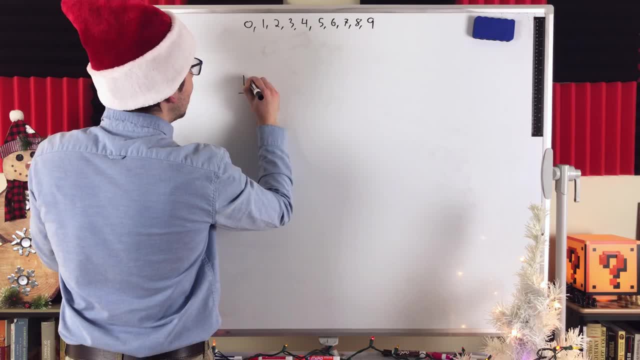 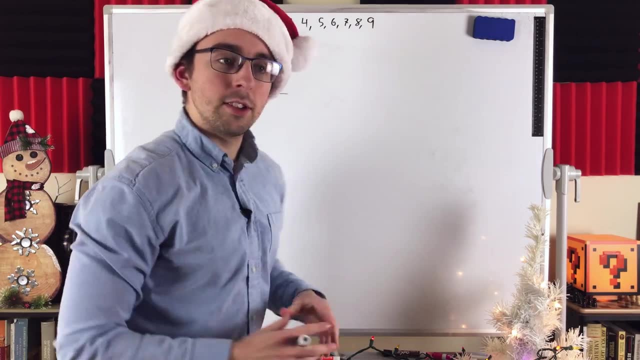 in our code and there are 10 possibilities. We could put any digit first, but things get a little different for the second number in our code. We no longer have 10 options, because whatever digit went first, we can't use it again because we're not allowing repetition. So now there are only. 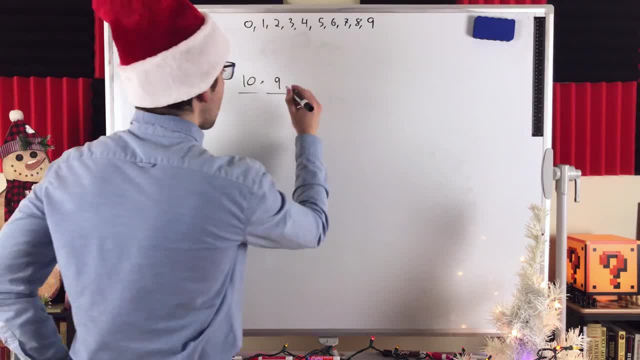 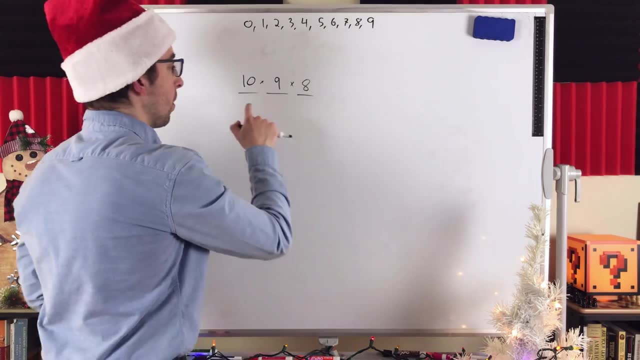 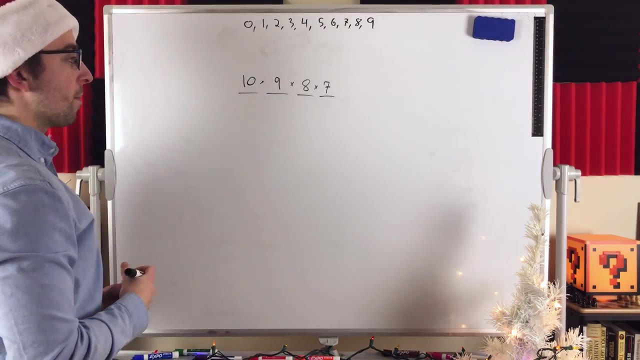 nine possibilities for the second digit, Then for the third digit, there are now eight possibilities left, because we can't use either of the two digits that were in these first two spots, And then for the last number in our code we've only got seven digits left to choose from. 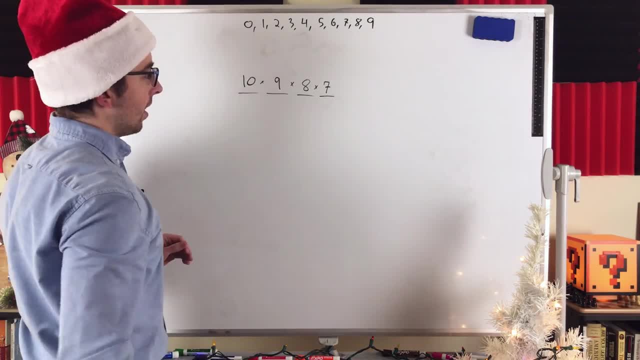 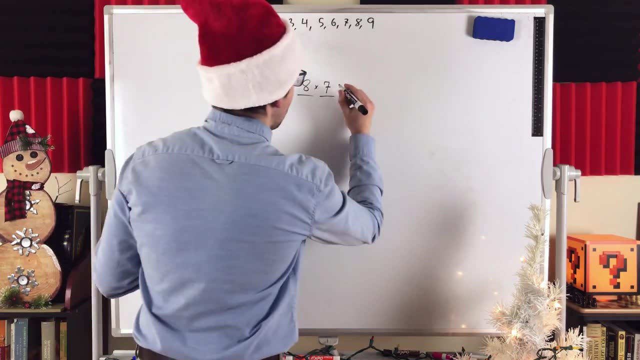 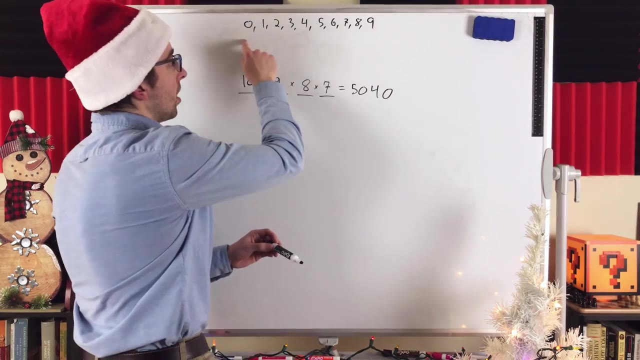 And so this totals up to, let's see: 10 times 9 is 90.. 90 times 8 is 720.. 720 times 7 is 5040.. So a total of 5. 40 possible four digit codes using the digits 0 through 9 and not allowing repetition. And in this, 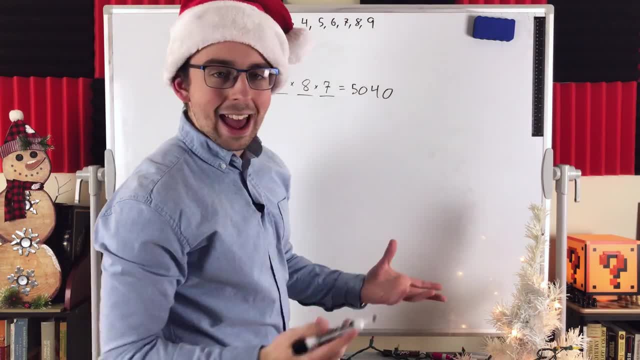 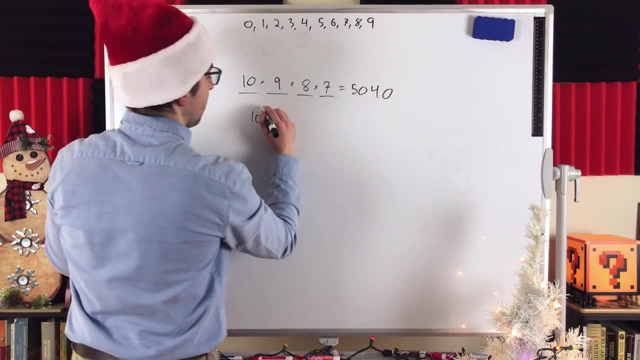 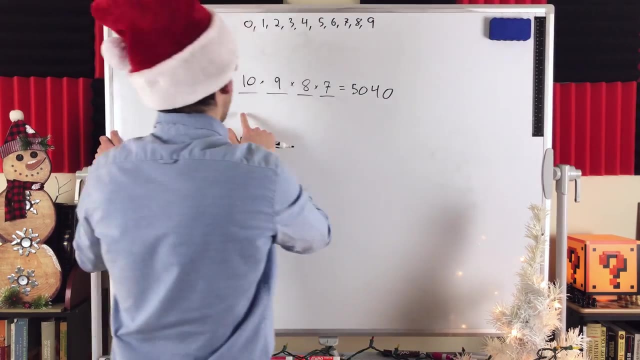 case, this turned out to be a little more than half of the total number of codes that could be created when we did allow repetition, which you might remember was 10 to the power of 4 or 10,000. So this is a little bit more than half of that. Now this could also be solved using what is called the 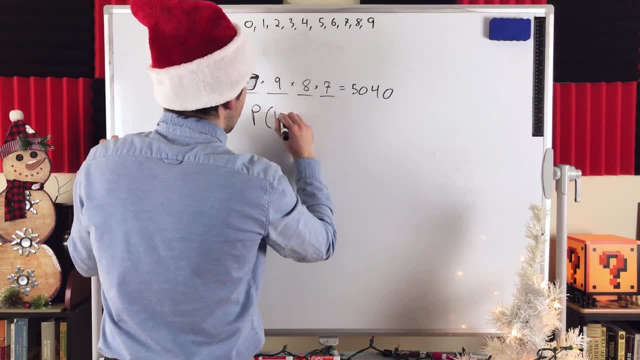 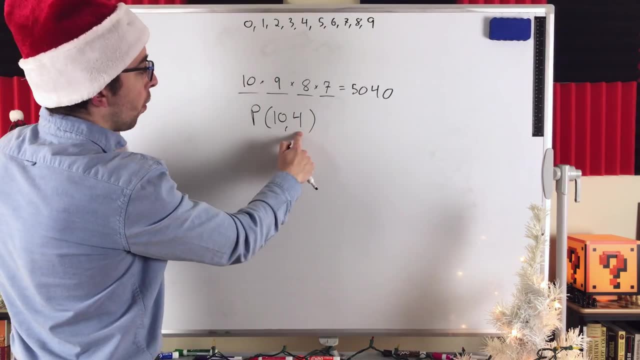 permutation formula often written like this. In this case it would be p of 10 comma 4.. This is the number of ways of ordering four objects: 1,, 2,, 3, 4- from a collection of n objects, which is what we've. 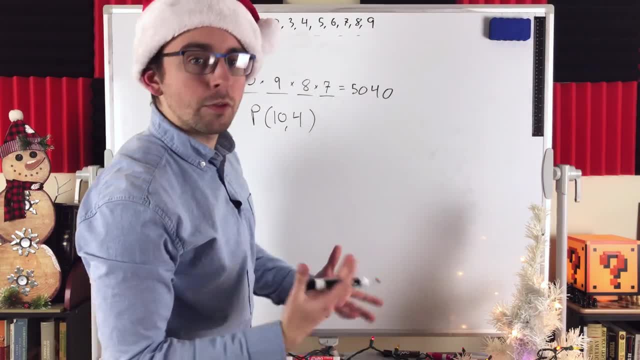 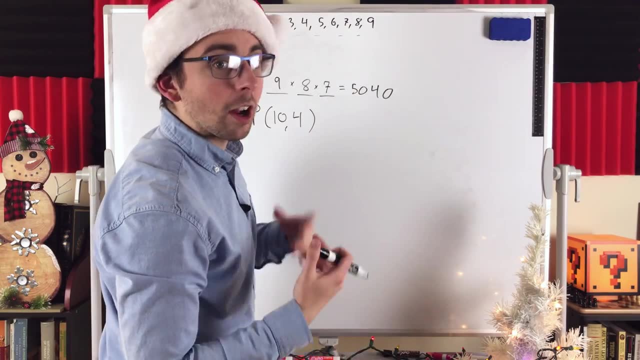 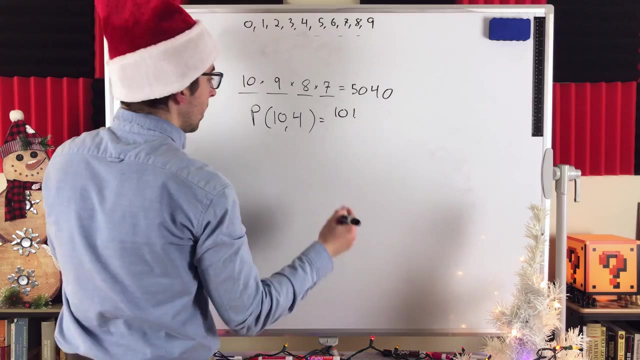 got here A collection of 10 digits and we're ordering four of them to create a code, And implicit in this formula is that repetition is not allowed. We're not allowed to use the same digit multiple times. So I'm just gonna say that the number of permutations of r objects from a collection of n objects is 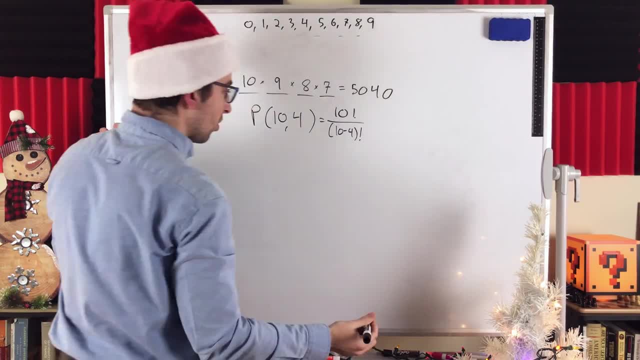 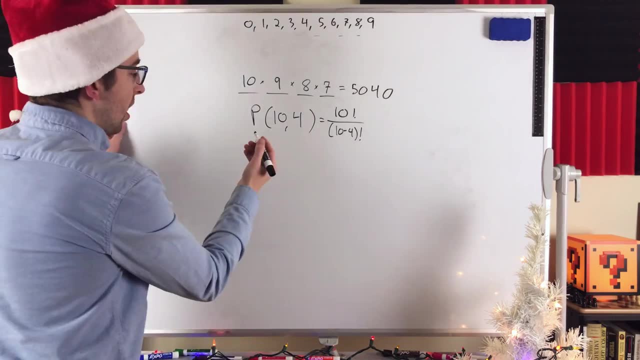 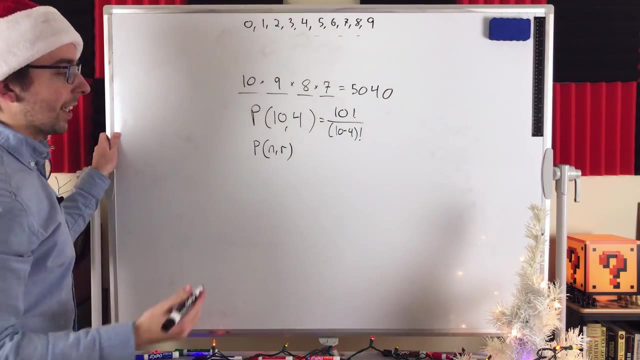 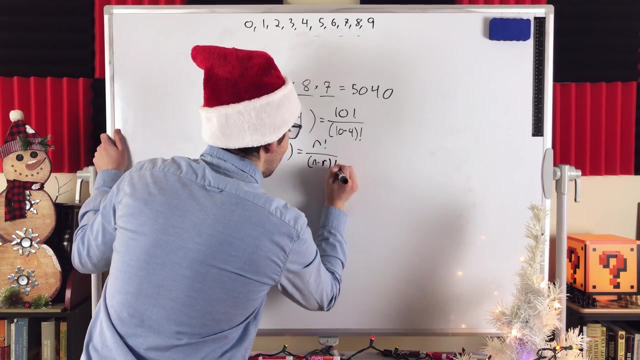 equal to 10 factorial divided by 10 minus 4 factorial Which, if you simplify these factorials, you'd end up with 10 times 9, times 8 times 7, of course, In general, of course, this formula- the number of permutations of r objects from a collection of n objects- is equal to n factorial divided by n minus. 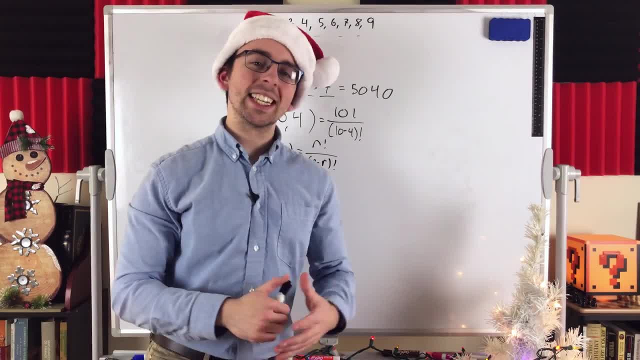 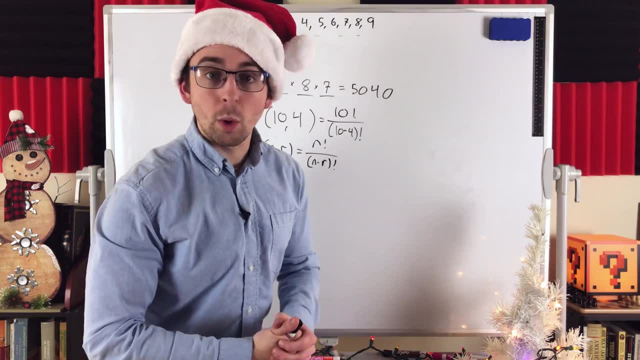 r, factorial, factorial, and i've got a pretty good lesson on that, so i'll leave a link to that in the description. you can go check out and see some more examples of this formula and a thorough explanation of why it works. all right, let's do just one more quick practice. problem with not allowing repetition. 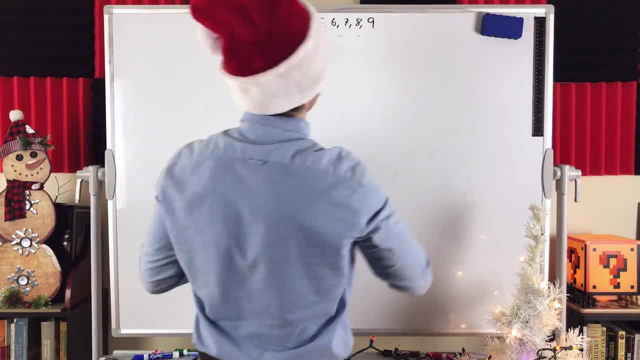 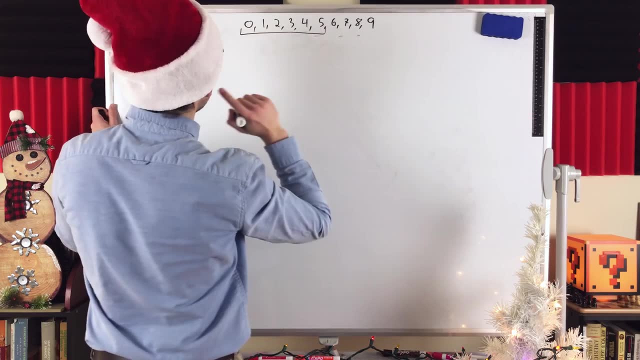 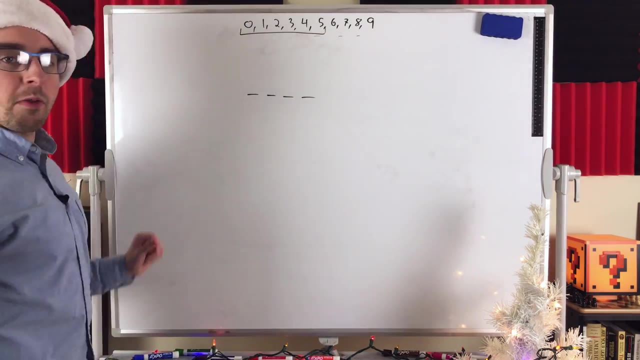 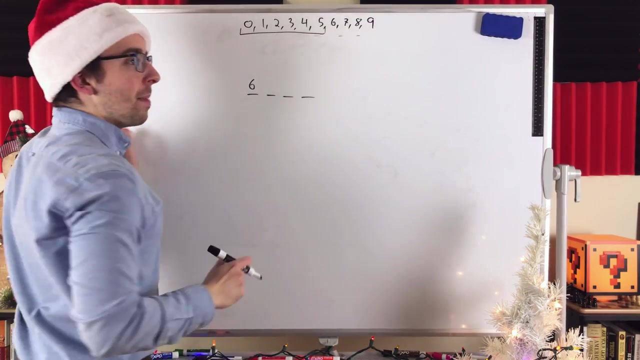 let's say, let's say we want to count the number of four digit codes we can create from the digits zero through five, not allowing repetition. so again, we're creating, we're creating four digit codes and we're not allowing repetition using these six digits. well, for the number that goes first, there are six possibilities. man, that plane is really loud. i. 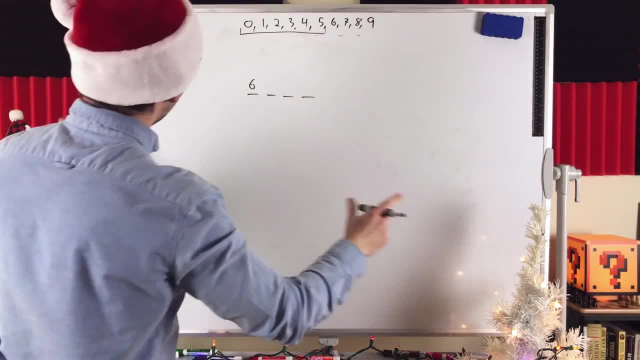 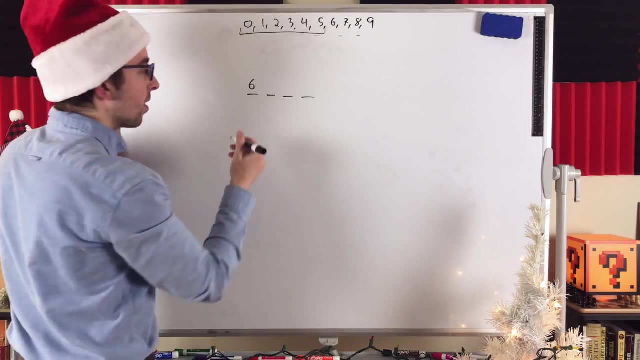 don't know how much the mic is picking it up, but it is loud for the uh. for the second digit there are five possibilities, because we can't repeat the digit that went first. so there's only five possibilities for the second number in our code and then similarly for the third number in our 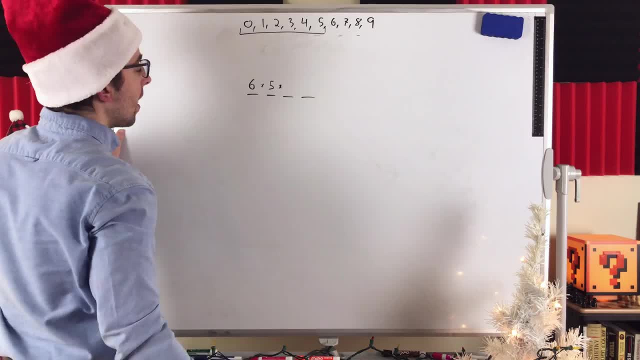 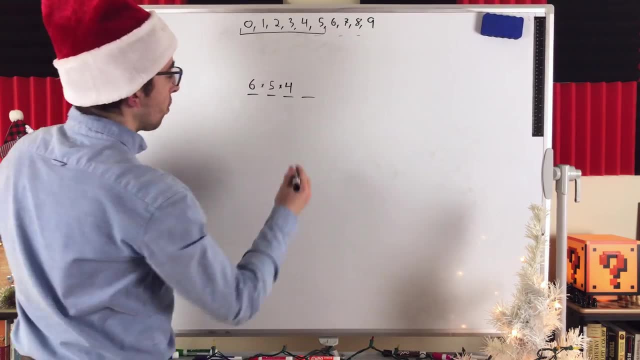 code. we had six digits to choose from originally, but we can't choose the first one again, we can't choose the second one again, so now only four digits remain to choose from, and then there's only third digits to choose from. for the last number in the code, this comes out to be six. 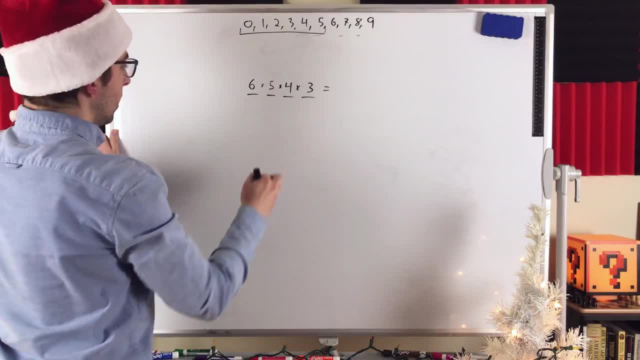 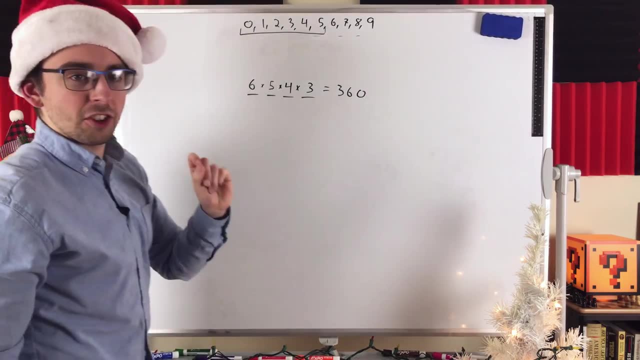 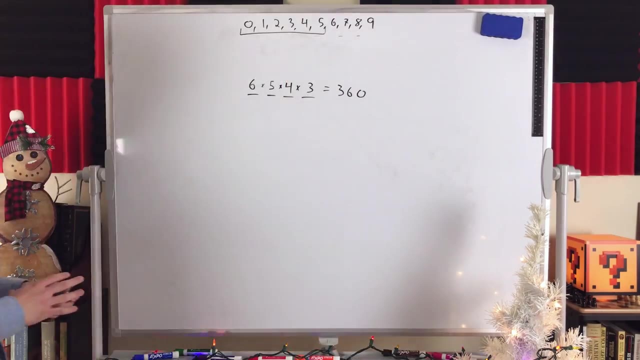 times five is thirty. thirty times four is one hundred twenty. one hundred twenty times three: that's the number of four digit codes that can be created using the numbers zero through five and not allowing repetition. so i hope these few examples helped you get a better idea of how.